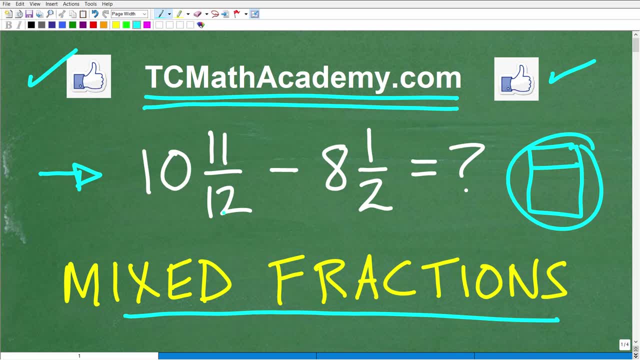 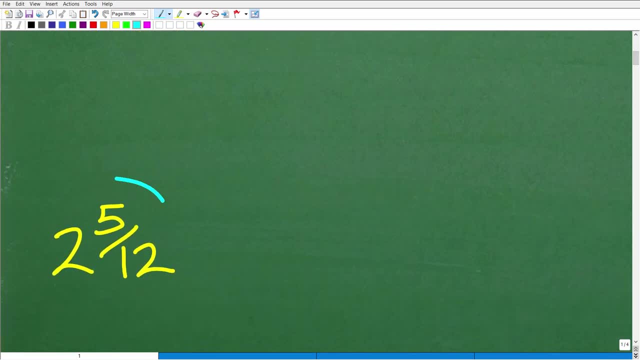 Okay, so let's go ahead and take a look at the answer here. So 10 and 11 twelfths minus 8 and 1 half. What is the correct answer? Well, the correct answer is 2 and 5 twelfths. 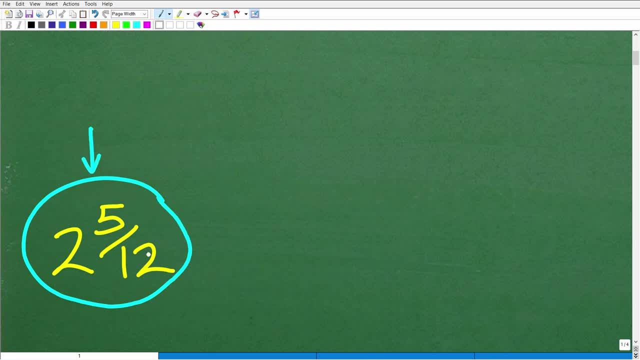 So notice that the answer itself is a mixed number. Of course you could write this as an improper fraction. Just a quick review. So if you have a fraction like, let's say 1 third, let's say 4 thirds and then of course, something maybe like 5 and 1 half, 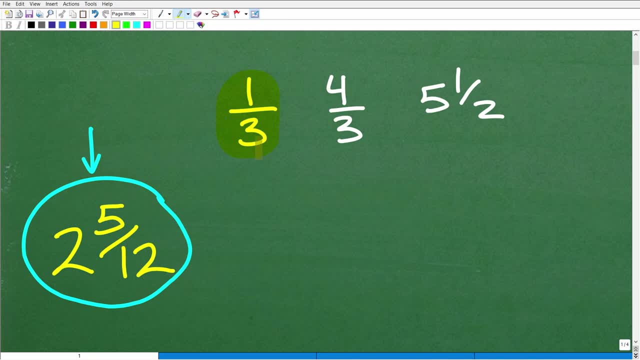 In mathematics a fraction like this is called a proper fraction because the denominator is a proper fraction. So if you have a fraction like this, let's say 1 third, let's say 4 thirds and then of course something maybe like 5 and 1 half. 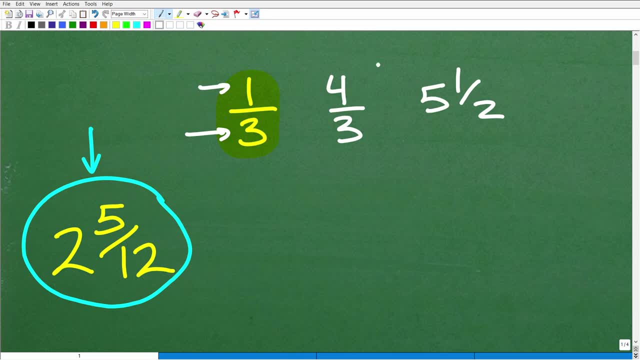 The denominator is larger than the numerator. Okay, Now, here the numerator is larger than the denominator, So we would call this type of fraction an improper fraction. Okay, so that's what this is called. And then, of course, this type of fraction is called a mixed number fraction. 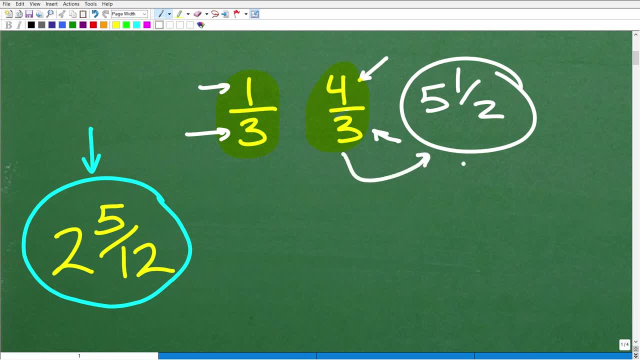 And you could convert improper fractions into mixed numbers and mixed numbers into improper fractions. That is a separate discussion, But anyways, we want to make sure we understand these proper terms In mathematics. But if you got this correct, that is fantastic. Matter of fact, let's give you a nice little happy face and a plus, a 100 percent and a few stars. 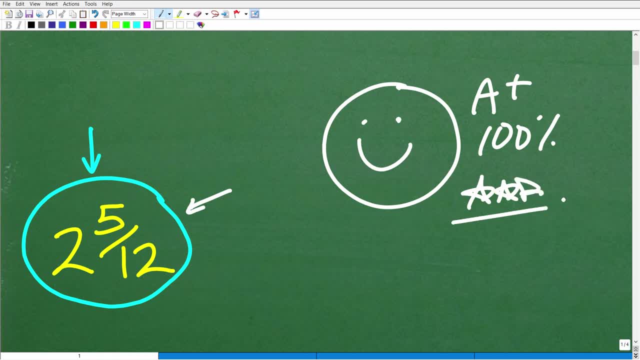 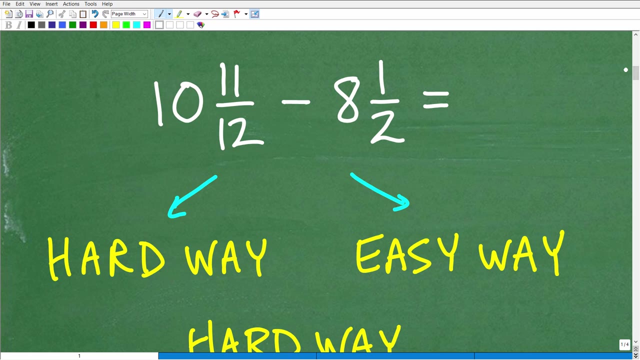 You could tell your friends and family that you know exactly how to subtract mixed number fractions. They'll be very impressed with that information for sure. All right, So let's go ahead and get into the problem And basically I'm going to go ahead and kind of categorize the way you can approach this problem as. 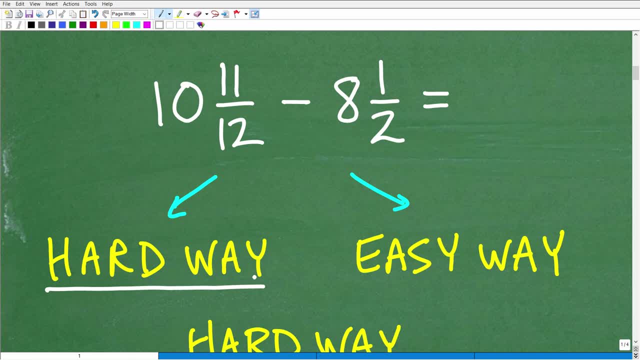 you have basically two options: You can do the harder way or you can do the easy way. Now, some of you might see this hard way. You'll be like: no, no, I like doing it that way And I got the right answer. If that is the case, that's perfectly fine. 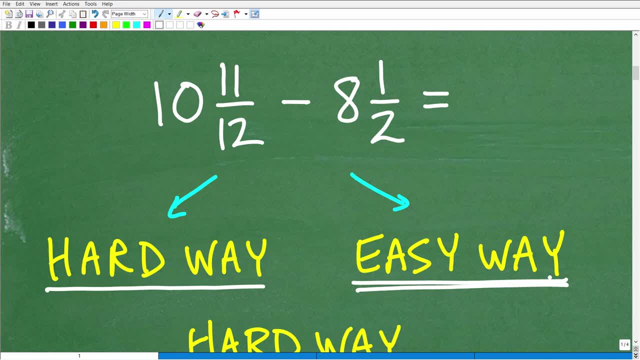 But in my opinion, this approach will be easier, And then, of course, this approach involves a little bit more number crunching, But either way, as long as you understand both techniques, that's what's important. Okay, And it is important to understand. 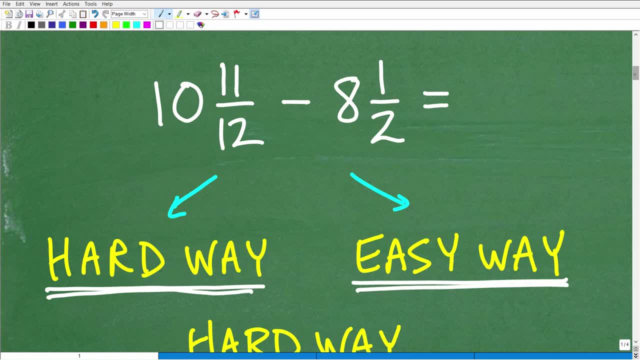 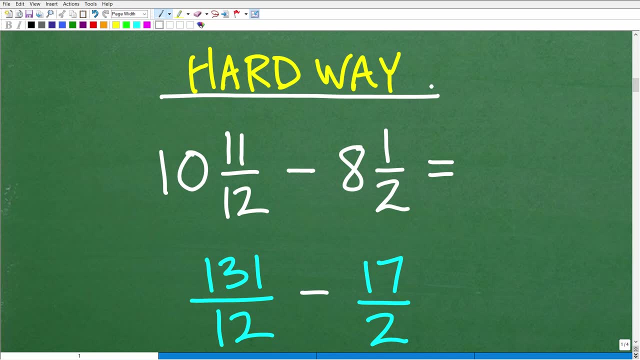 Both approaches to doing this problem All right. So let's go and get into this right now. So what I would say is the hard way to approach this problem is to turn these mixed number fractions into improper fractions. In other words, here we have 10 and 11 twelfths. 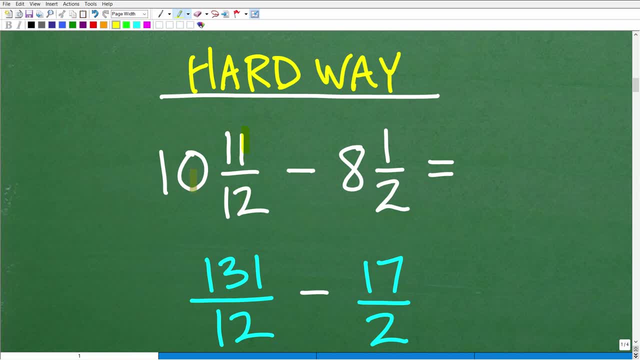 So if I wanted to write this again, this mixed number, into an improper fraction, I would go 12 times 10.. That's not too bad, Right? So 12 times 10.. That's 120.. Then you're going to take that 120 and add 11 to it. 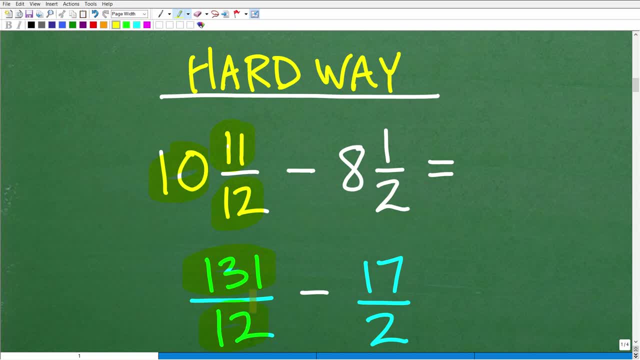 So you're going to have 131 over 12.. So now you know it's a little bit extra work. These numbers are this 10 here obviously makes this multiplication pretty easy. But then we got to do the same thing here. 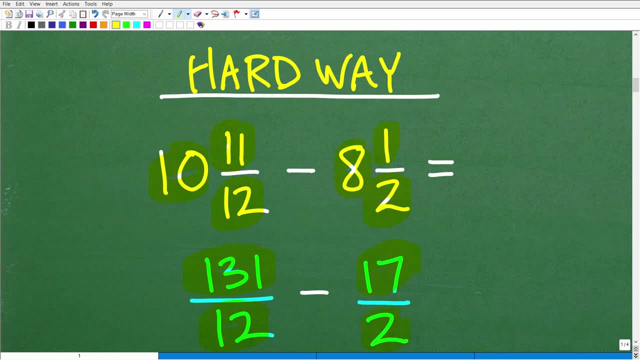 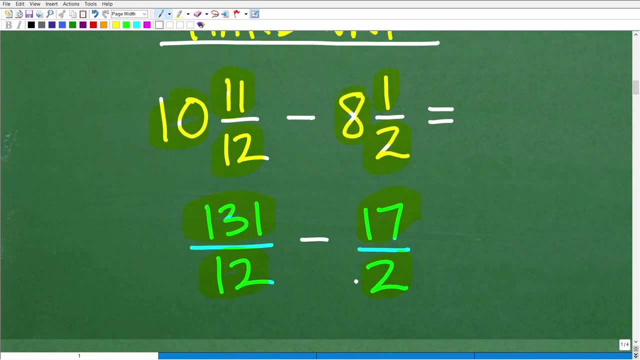 So we have two times eight, That's 16 plus one. So this would be 17 halves. So this is what I would say is a little bit of the harder way. Now, in this particular problem we don't have common denominators. 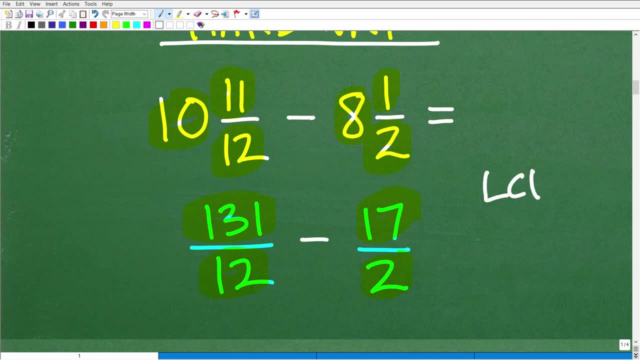 So we would have to find the LCD. Hopefully you recognize the LCD. here is 12.. So to fix this up, we just simply have to multiply this by six and then 17 by six. So we'd have to do some multiplication here and then we would have to track the difference. 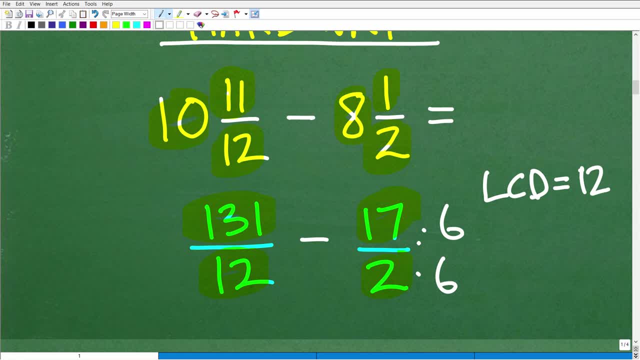 Right. So this is one approach to doing this problem. OK, Now, another approach All right- Is what I'm going to classify as the easy way. Now, if you did the problem this way, that's perfectly fine, And you do need to understand how to do, how to write mixed number fractions into improper fractions and do a problem like this. 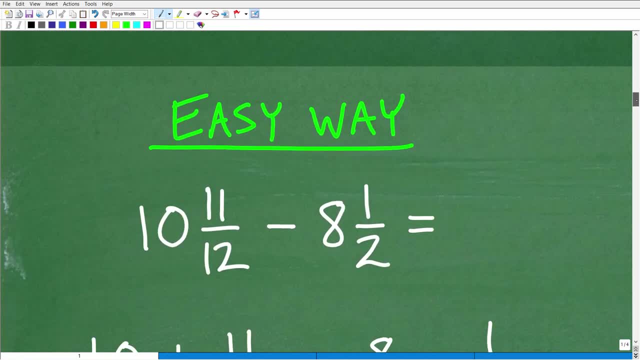 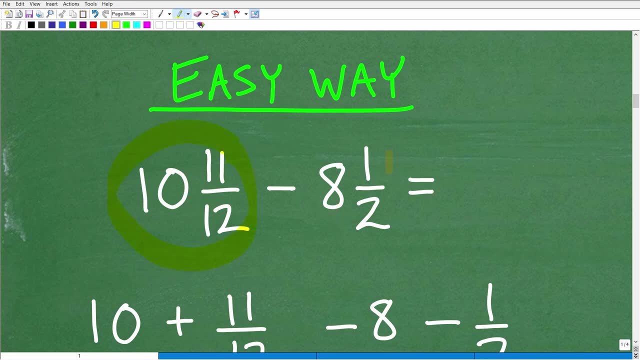 Right. But let's see another way we can handle this problem, because we are dealing with mixed numbers, All right, So we have a mixed number fraction. We need to kind of conceptualize each one of these numbers. OK, so 10 and 11, 12.. 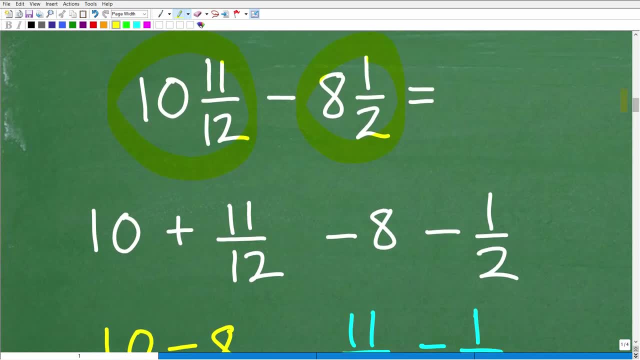 So let's talk about what a mixed number means. Well, this means 10. Plus 11, 12.. So we can really think of it as 10 plus 11, 12.. That's what this value is right here. 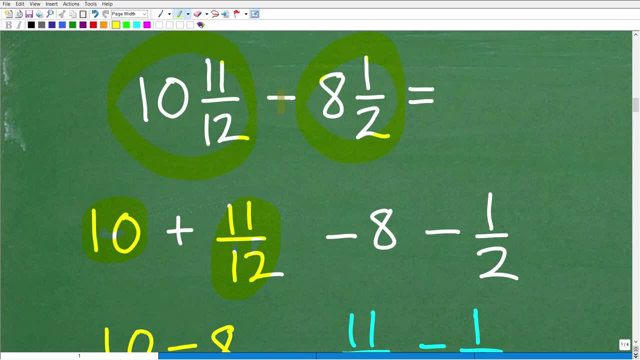 10 plus 11,, 12.. Now we're taking away. We're going to subtract away eight and one half. So we've got to subtract an eight away, And then we also got to subtract a one half away. So in total we want to subtract eight and one half. 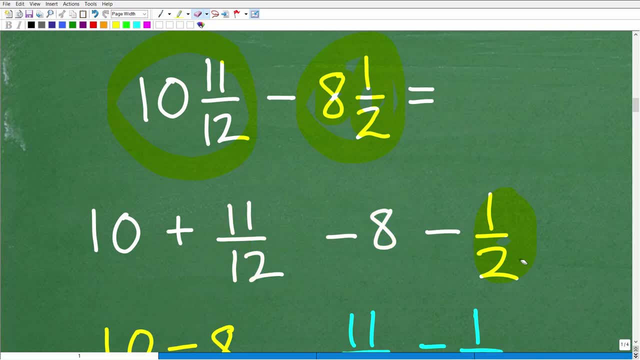 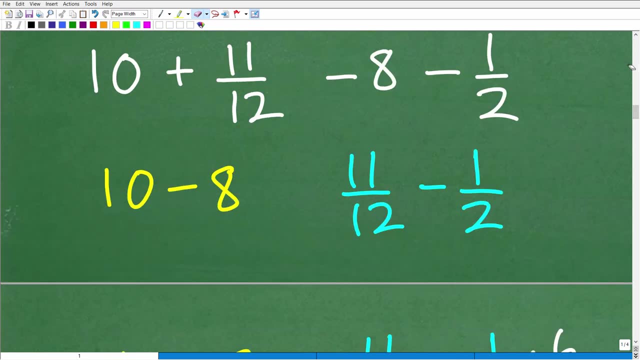 So if you look at the problem this way, OK, you can kind of shuffle these numbers around And make this problem much easier, OK, so again, we kind of go back up here. So we're going to think of 10 and 11, 12 as 10 plus 11, 12.. 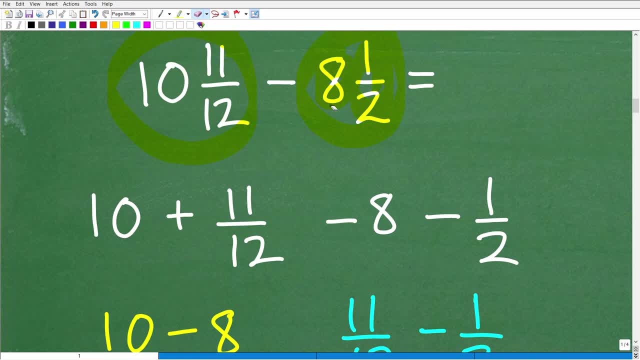 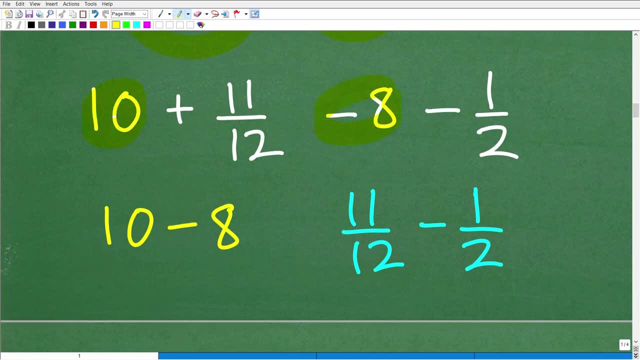 And we're going to take away eight and another one half, or total of eight and one half. So when we do this, let's just go ahead and grab these easy numbers: 10 and minus eight, Right. So 10 take away eight, or 10 minus eight is right here. 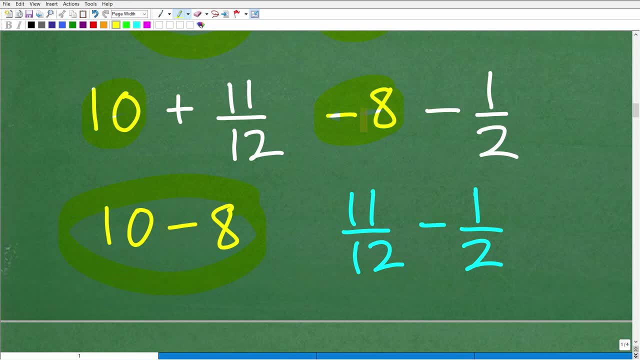 Of course, we know that that's going to be two, So we can kind of basically add up all of them, Add up all these numbers, But when it comes to adding numbers, the order is important. OK, like one plus three plus four is the same thing as one plus four plus three. 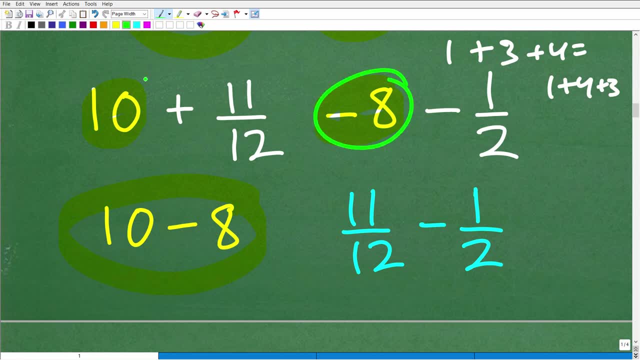 OK, but then what we can do, we could take care of these two right here, Right Get the answer. Of course we know it's going to be two, And then what we really have to just concentrate on is 11 minus one half. 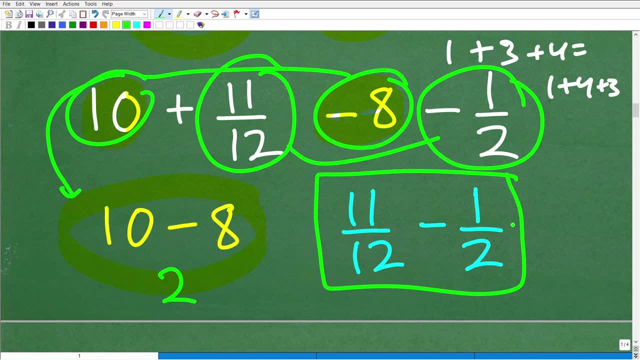 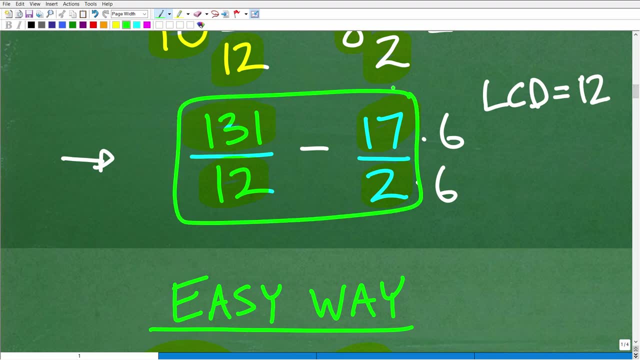 So dealing with this fraction right here, Or this subtraction problem, is much easier than to deal with this fraction problem here Again, we don't have a calculator. You know we don't want to use a calculator. So now let's go ahead and finish this problem up. 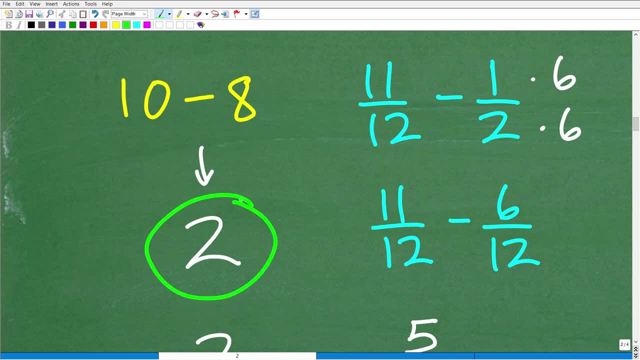 All right. So again, 10 minus eight will be two and 11, 12 minus one half. Of course, we don't have common denominators. The common denominator, or the lowest common denominator, is 12.. So all we have to do is multiply this denominator by two to get a 12.. 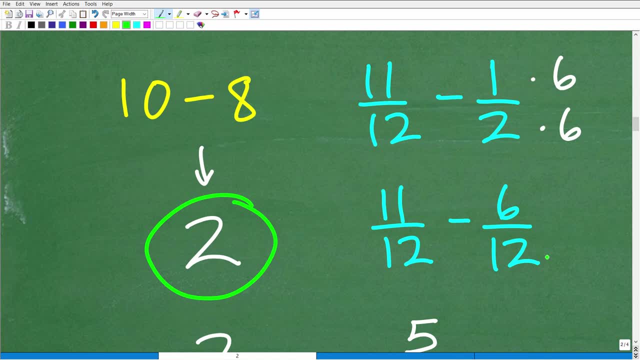 I'm sorry. a six To get a 12.. So six times two is 12.. And then when we multiply the denominator by six, we've got to multiply the numerator by six as well. So now we have 11 twelfths minus six twelfths. 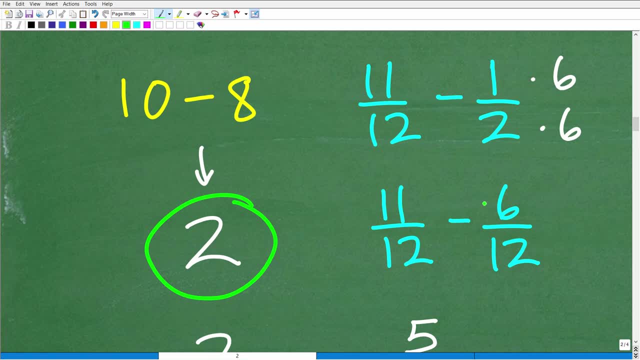 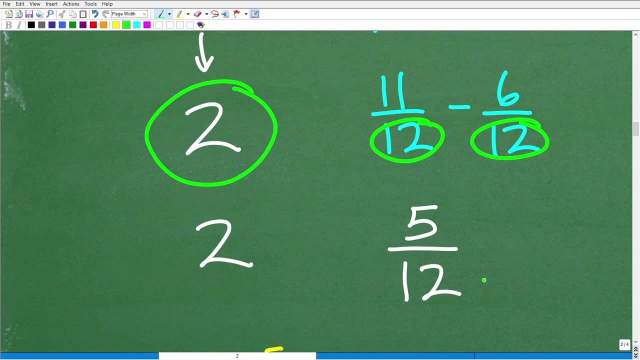 OK, And of course six twelfths is the same thing as one half, And now we can simply subtract the numerators, Right? So we're talking about basic subtraction of fractions. So we keep that same denominator- 12, and we subtract the numerators. 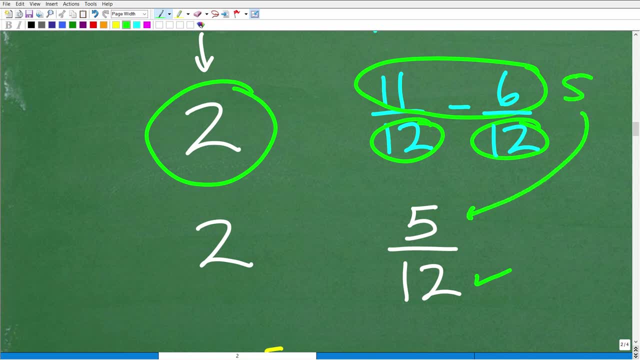 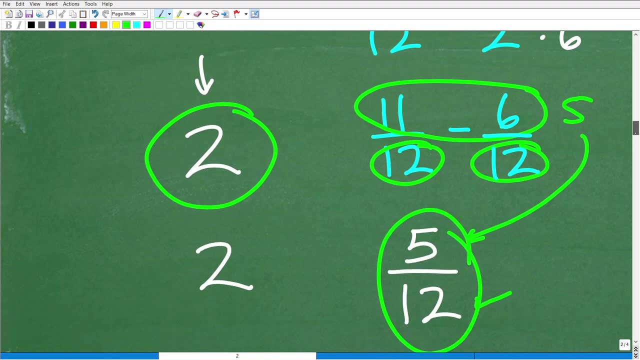 11 minus six is five, So this will be our answer here. So this part is five twelfths, And we already answered what 10 minus eight is. That's two. So this is two and five twelfths. Or we could write it just like this: two and five twelfths. 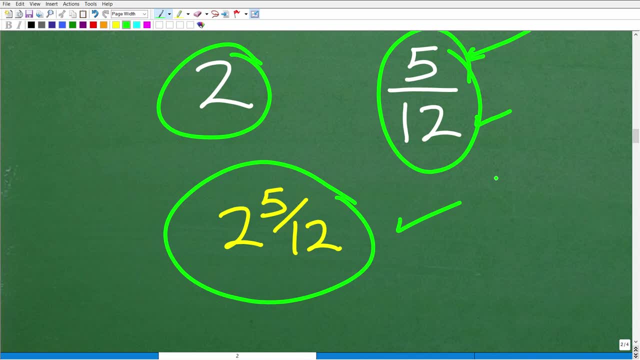 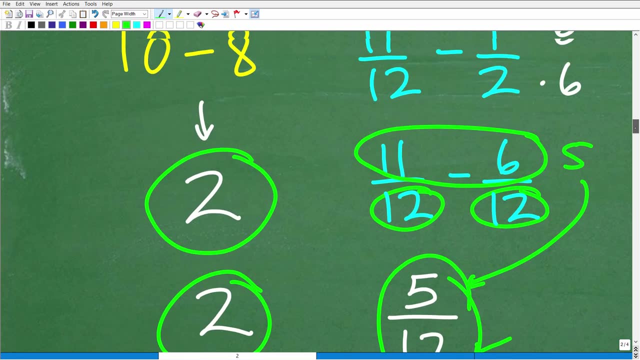 Now some of you might be saying: well, that was like a lot of explanation, That's like a lot of, that's like a lot of work. You actually did the hard way. The other way was easier. Well, it seems it might seem a little bit harder because I'm explaining it. 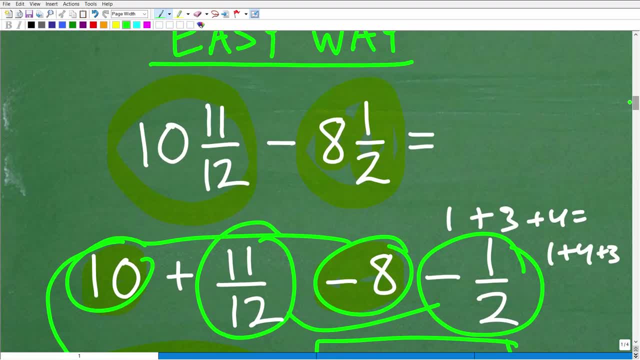 You know I'm kind of explaining the process here, But the main idea is You got to realize that these mixed numbers you could break them up into two separate like numbers: 10 and 11 twelfths. It's the same thing as 10 plus 11 twelfths. 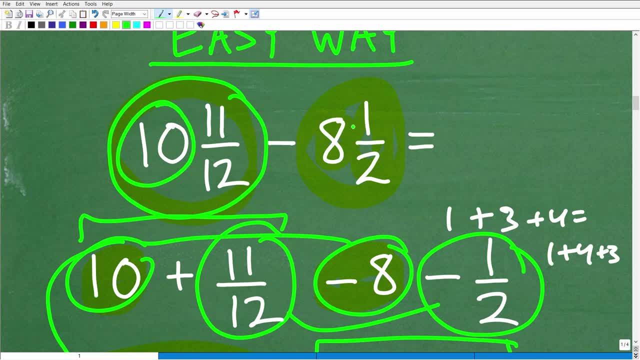 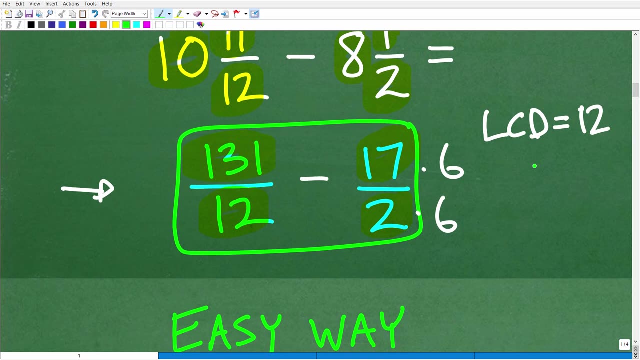 OK, and that way you can handle these big whole number parts, these big integer parts. Take that out of the equation. I just do the math there and deal with simpler fractions. This is a more user friendly approach, especially when you don't have a calculator, because here you're going to have to do some side multiplication. 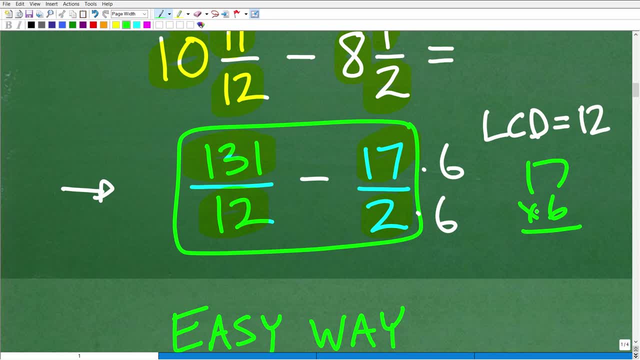 17.. 17 times six. and then you have to do some subtraction And fortunately, in this particular problem it's easy to find the LCD. It's simply 12.. So here I just have to multiply by six. But let's say I had to multiply both of these fractions to get the lowest common denominator. 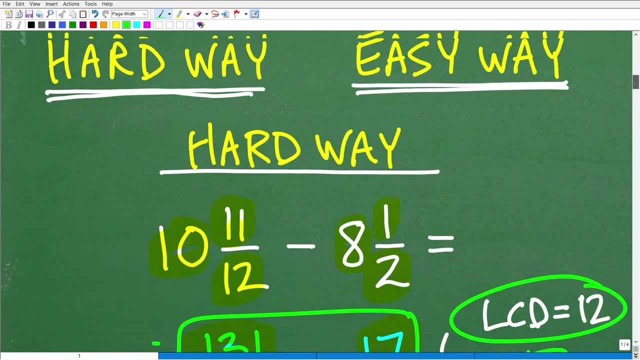 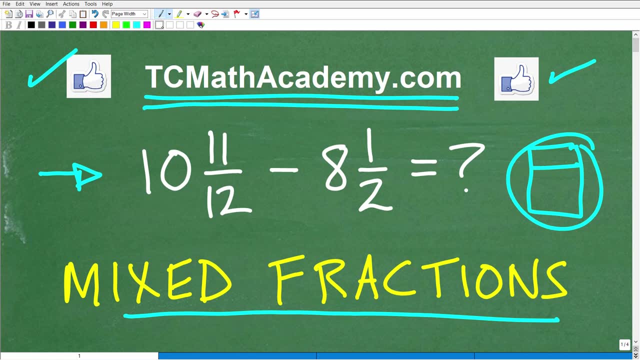 Then I multiply by 131,, et cetera, et cetera. So, anyways, if you need additional help with fractions or arithmetic or basic mathematics, let me give you a couple of suggestions. One: I've got a ton of videos on my YouTube channel on fractions and basic mathematics. 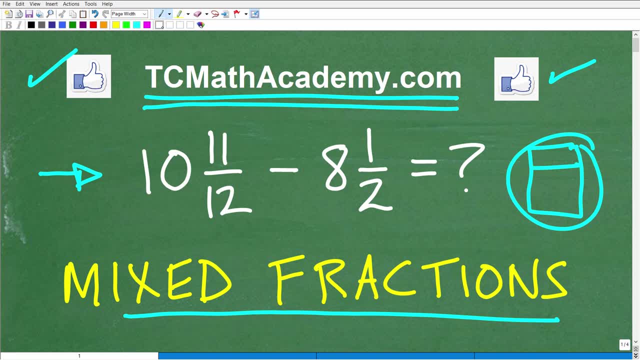 But if you're looking for a more kind of formal way to build up your basic math skills, check out my math foundations course. Of course you can find that at TCMathAcademycom. It is a great little, it's actually a very popular course.